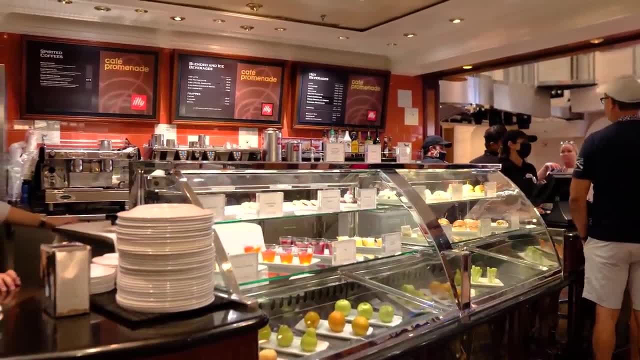 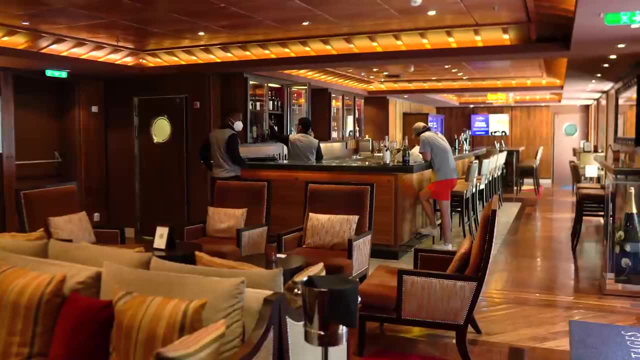 Purchases and services rendered on board a Royal Caribbean ship will have gratuities added at the time of purchase. If you buy a drink, get a massage at the spa or eat at a specialty restaurant, you'll be charged an 18% gratuity automatically. There's nothing else you have to do extra. 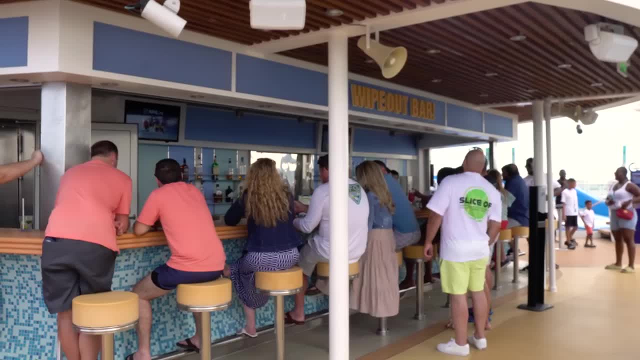 and the gratuities will be charged at the same time. If you buy a drink, get a massage at the spa. the cost breakdown will be on your receipt. Drink packages and specialty dining packages will be charged an automatic gratuity upon purchasing the package, which means 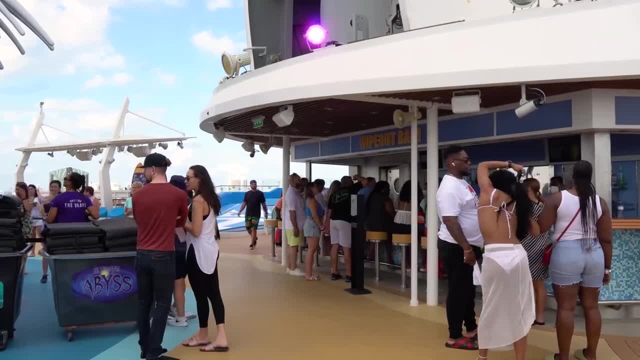 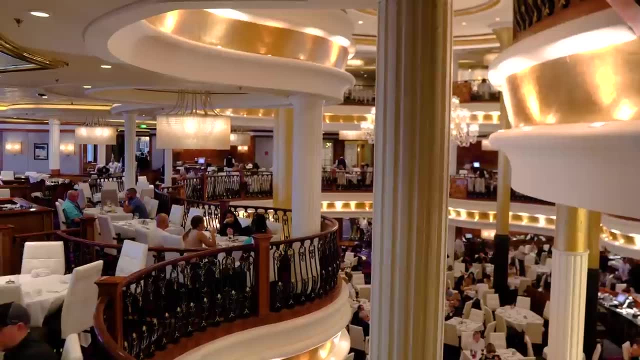 no additional gratuities required when taking advantage of the package. benefits like ordering a drink at the bar with a drink package as an example. Now, beyond all that, there are opportunities to give crew members an additional tip for excellent service, as you see fit, Even. 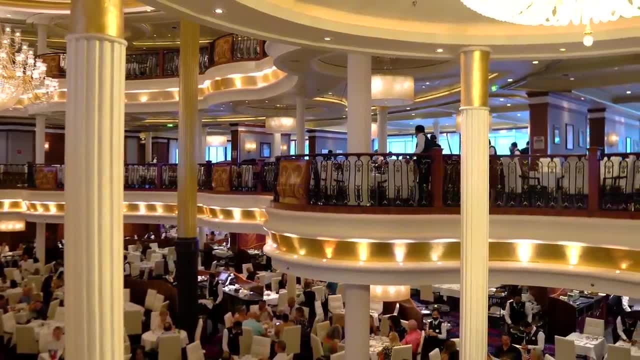 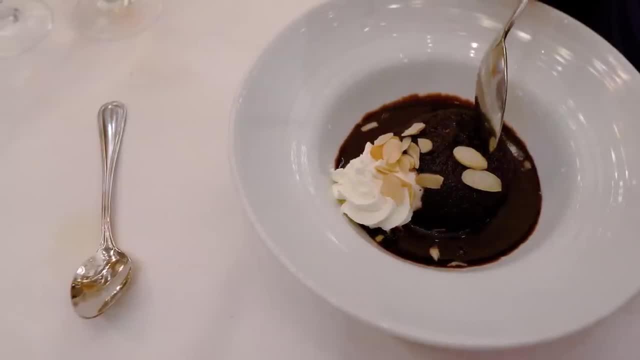 crew members who receive an automatic gratuity can receive additional gratuities if you feel it's warranted, and that really comes in the form of, you know, opting to give them a dollar here, a dollar there. Let's move on to the most common question about what's included, and that is meals. 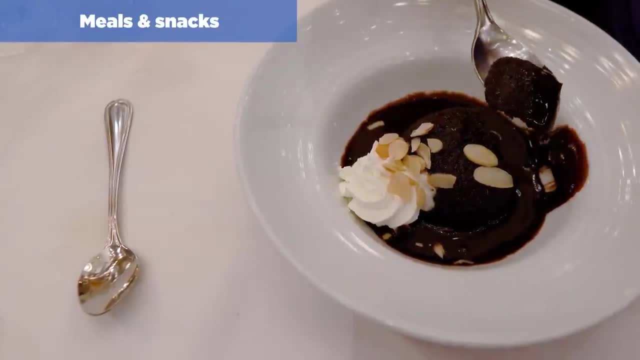 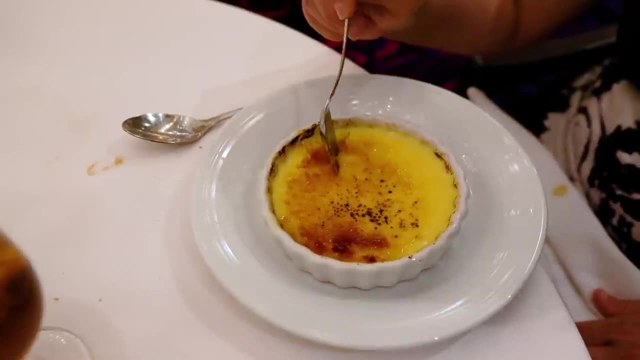 and snacks. All Royal Caribbean cruise fares include most meals and snacks on board your ship, at any private destination that you visit, like Labadee or Perfect Day at Cocoa Key. This means there will be ample opportunity to enjoy breakfast, lunch, dinner and snacks without any additional. 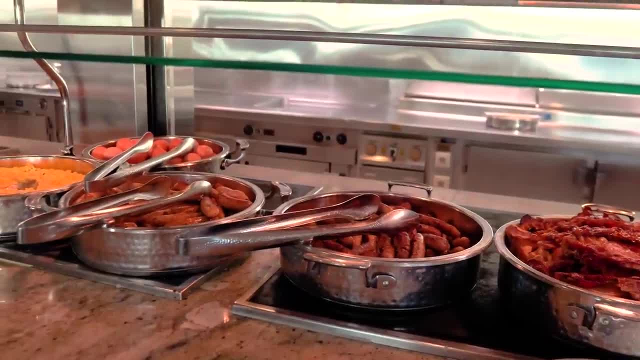 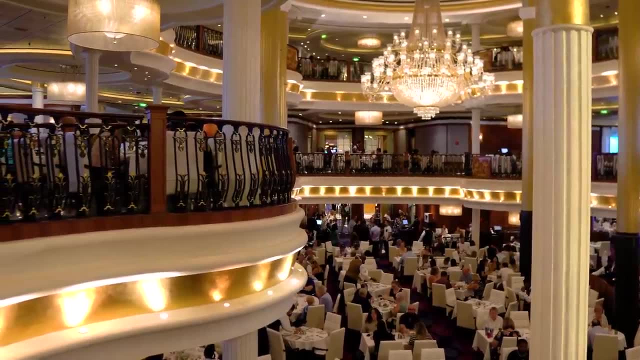 cost. Now, the exact venues included with your cruise fare will depend on the ship you're sailing on, but here are some venues that are pretty much found on nearly every Royal Caribbean cruise ship. The main dining room, which is the hub of dining on a Royal Caribbean cruise, is open for breakfast and dinner every day. 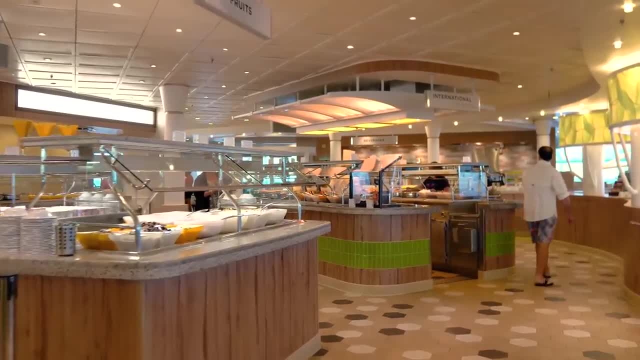 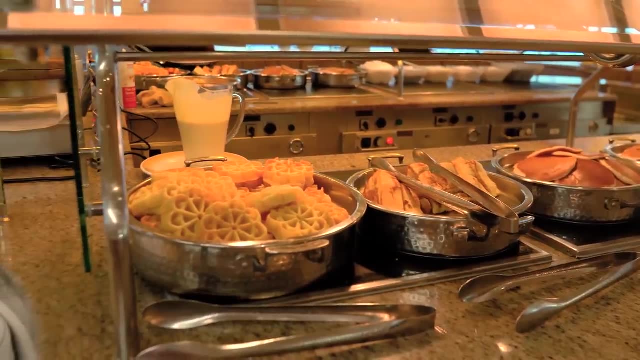 and for lunch on sea days, The Wind Jumeirah Buffet is included as well. This is Royal Caribbean's signature buffet, featuring a wide assortment of cuisines, dishes and flavors. It's open for breakfast, lunch and dinner every day. On some ships you may have the Solarium Bistro, which is 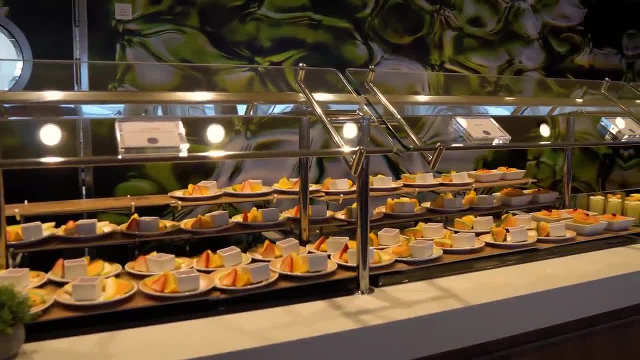 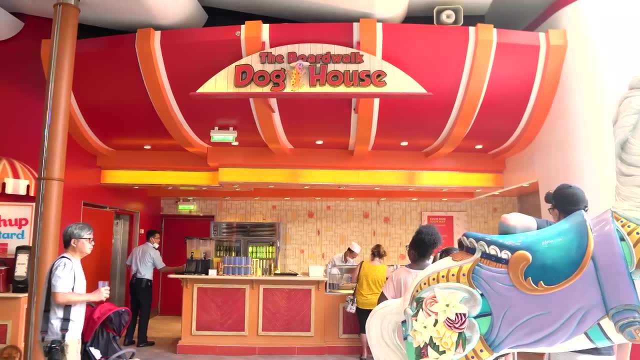 a Mediterranean-style restaurant open for breakfast and dinner on Oasis and Kwan Kla ships. Grab-and-go spots for foods such as Café Promenade, El Loco Fresh, Sorrento's Pizza, Boardwalk, Doghouse Park Café, Café 270.. These are all casual venues with quick-service meals and the selection of. 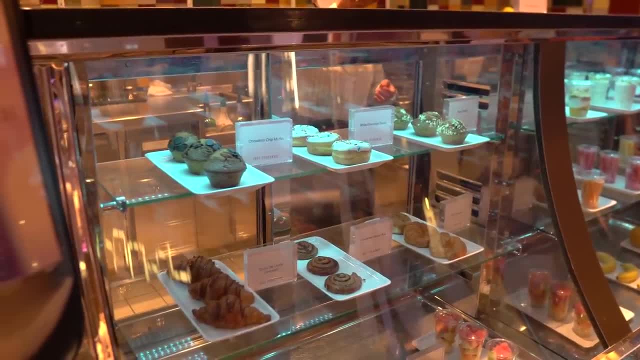 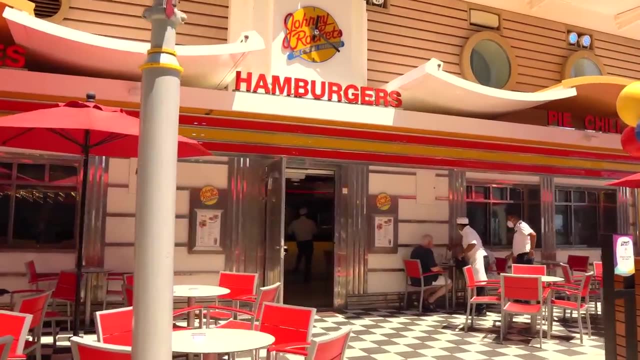 grab-and-go venues changes by ship, but this is all included, And if you happen to sail on an Oasis-class ship only, then Johnny Rockets is included for breakfast only. For lunch and dinner it still costs extra. There are an extensive amount of complimentary dining options on a Royal Caribbean. cruise, so it's pretty easy to go an entire cruise by eating only at restaurants included with your cruise fare Plus. Royal Caribbean maintains excellent food quality and you don't have to call in all of its dining venues- complimentary or specialty. You may find a few extra-cost items. 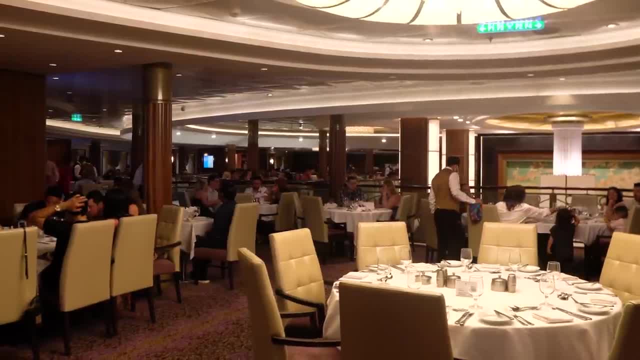 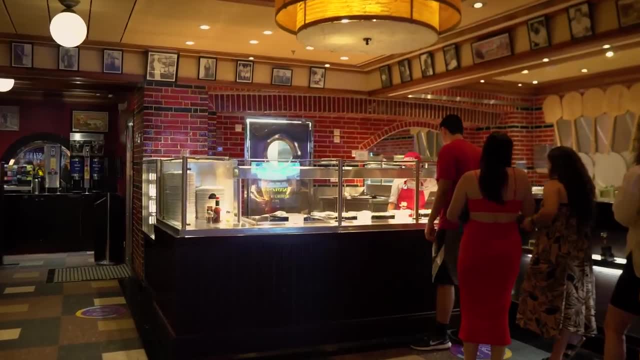 in the main dining room, such as filet or lobster. These items are available for free on cruise ship formal nights during your cruise, but come at an extra cost on other nights. Royal Caribbean offers its guests pizza at some of its restaurants and buffets, as well as Sorrento's on the larger 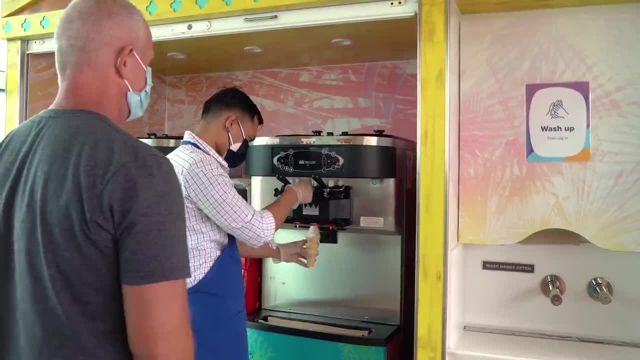 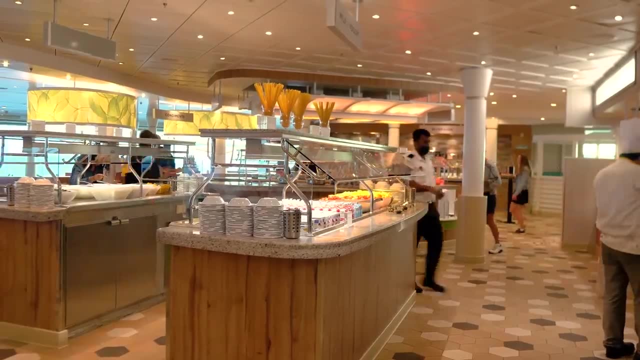 ships. Pizza at these locations are included with your cruise fare. Soft-serve ice cream can be found near the pool deck and is in operation for most of the day and included as well. The Windjamere and main dining room also offer their own selection of hand-scooped ice cream. 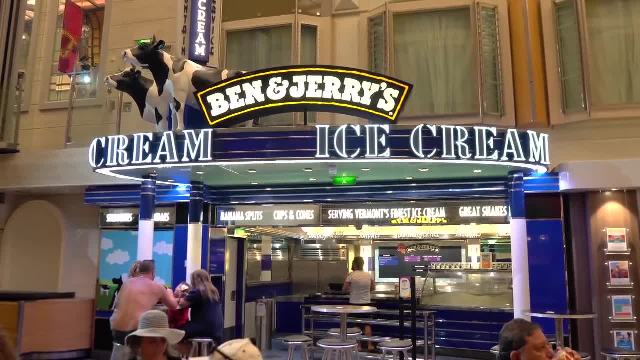 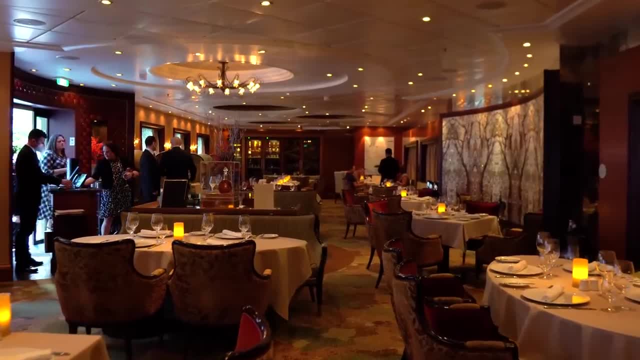 some Royal Caribbean ships even offer Ben and Jerry's ice cream, which does come at an additional cost. Let's talk about things that do cost extra in terms of food and drink on board your cruise, Of course, in addition to all the complimentary dining I talked about Royal Caribbean offers. 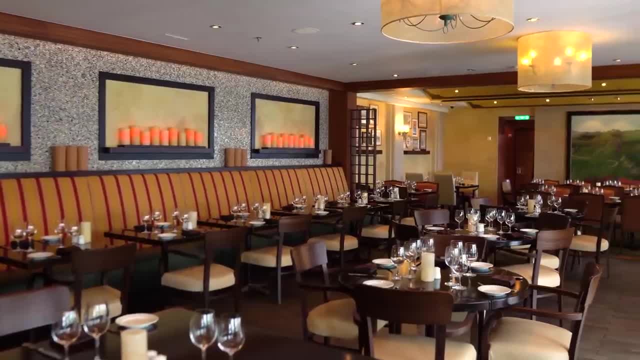 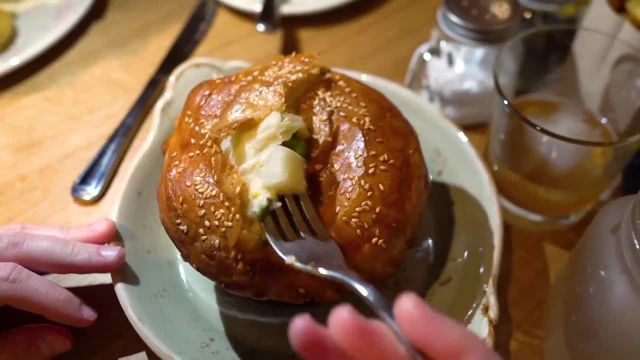 specialty dining, which comes at an extra cost. Specialty dining allows either a cover charge or a la carte. pricing depends on the restaurant. Now here's a list of specialty restaurants in Royal Caribbean's fleet. Specialty restaurants vary per ship, with some smaller ships offering. 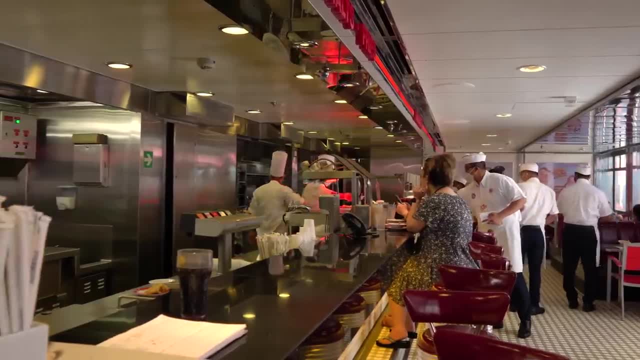 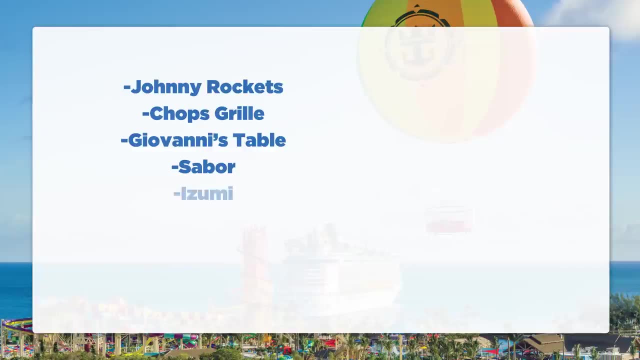 maybe two or three specialty venues, whereas larger ships can offer up to seven or eight different restaurants. So here's a list: Johnny Rockets, Chop's Grill, Giovanni's Table Sabor, Izumi Hibachi and Sushi. Jamie's Italian Sampa Grill. 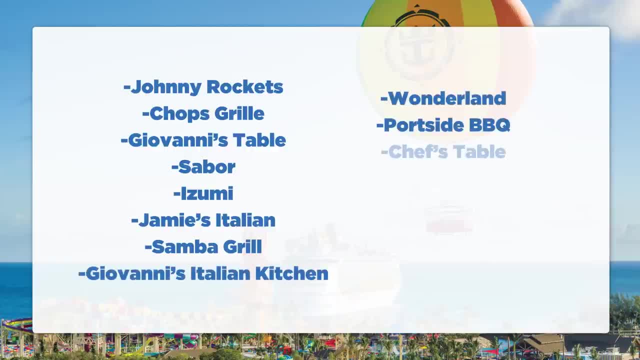 Giovanni's Italian Kitchen, Wonderland, Portside Barbecue, Chef's Table, 150, Central Park, Hooked Seafood, Playmaker's Sports Bar and Arcade and The Mason Jar. The reason to indulge with a specialty restaurant is because it offers cuisine options not otherwise available on your ship. 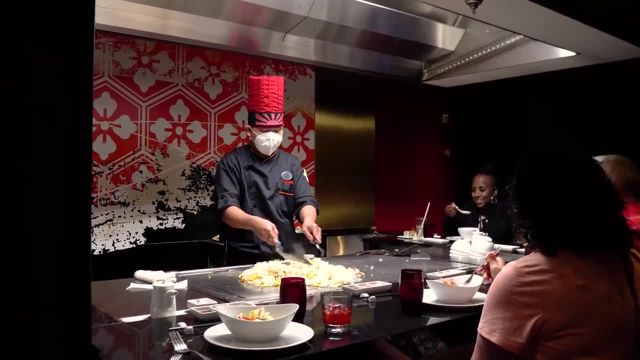 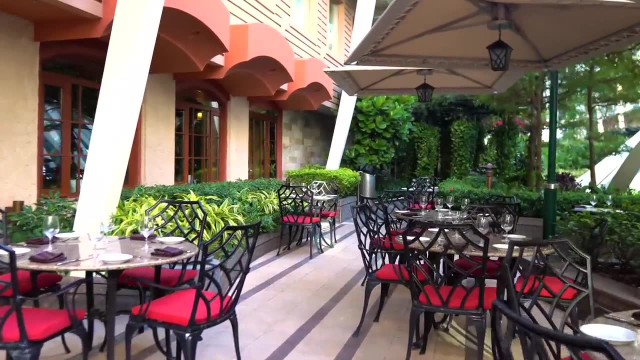 as well as the opportunity to enjoy the food and drink meals that you may prefer to enjoy at your own pace. In addition, the ambiance is usually enhanced at these locations and the prices charged are not exorbitant, Even though Royal Caribbean's. 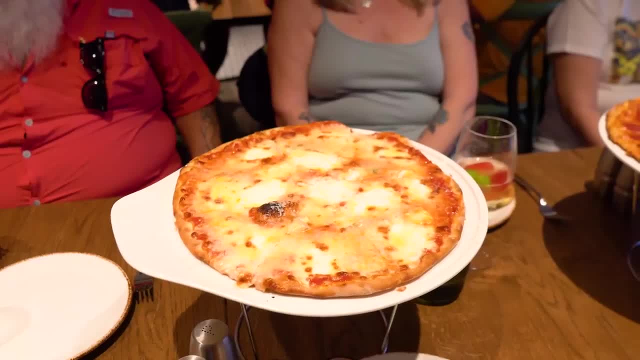 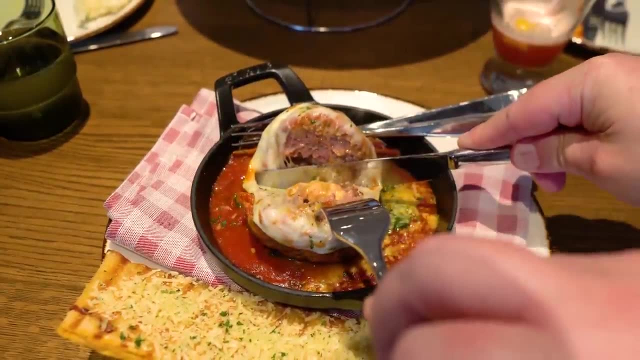 complimentary dining options are very good. specialty restaurants can be a great way to enhance or splurge on your cruise. Dining at a specialty restaurant can also be a nice way to celebrate a special occasion. All right, let's talk about drinks that are included and cost. 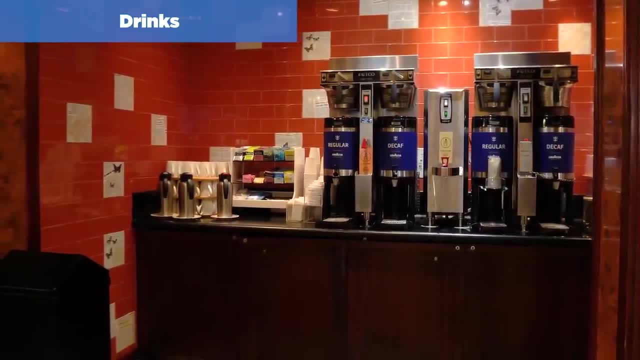 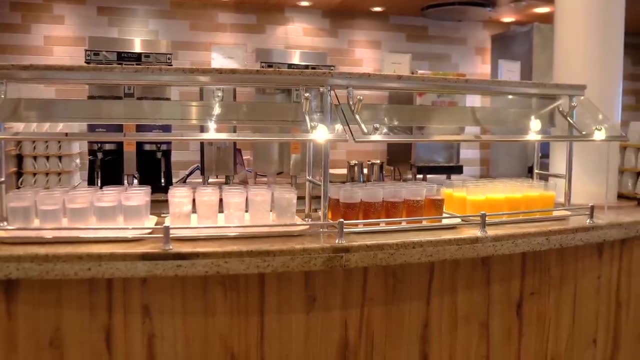 extra on a Royal Caribbean cruise. Royal Caribbean provides a selection of beverages included with your cruise fare, and these drinks are available at any time and include tap water, tea, coffee, lemonade, iced tea, milk, juices that are not fresh squeezed and hot chocolate. 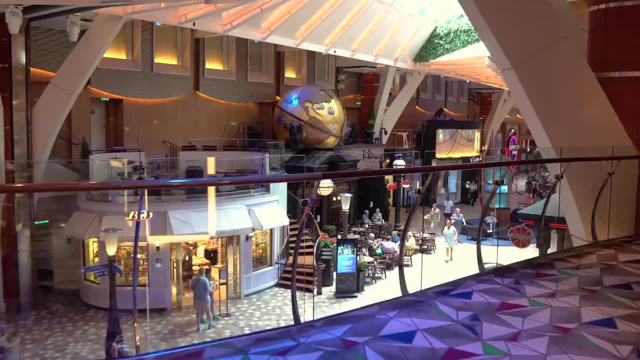 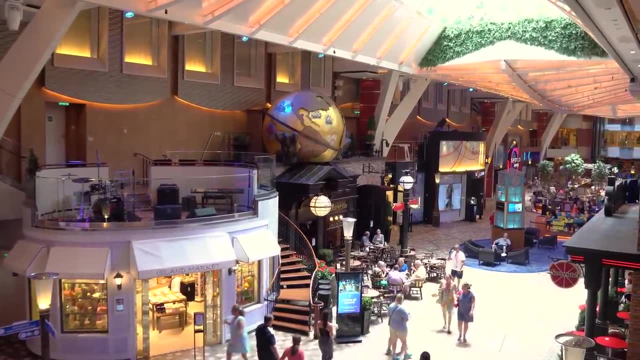 These drinks I just mentioned are available on board at a number of locations, such as Cafe Promenade and the Wind Jumeirah or Main Dining Room. Water can be found at any bar on board as well, and it's safe to drink the tap water on board, as it's really of high quality and probably 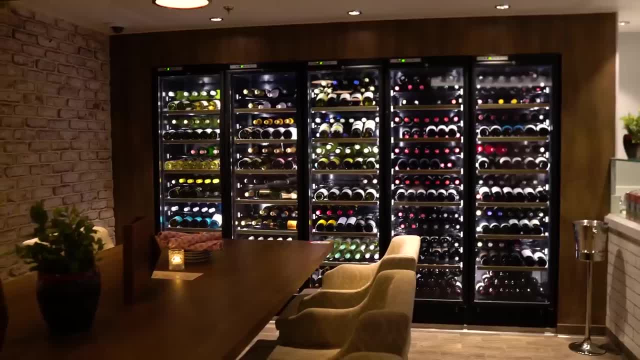 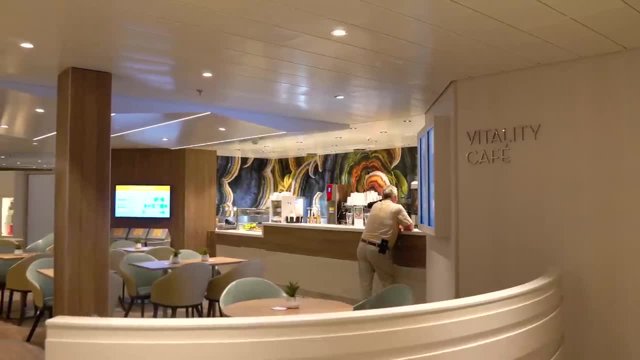 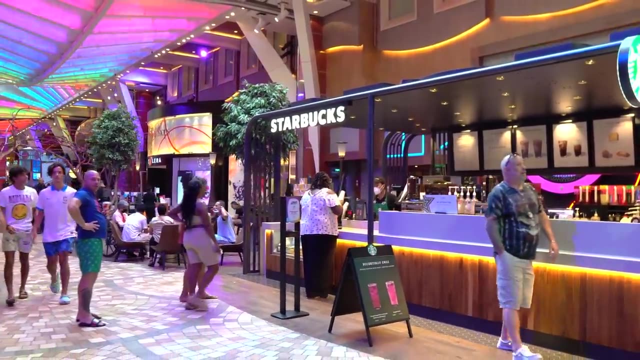 better than any tap water you can find back at home. Alternatively, if you want beverages like alcohol, soda, fresh juices, mocktails, specialty coffee drinks, milkshakes, canned water and Starbucks beverages, you can purchase them for an additional cost during your cruise. Now Royal Caribbean offers you the option when it. comes to these drinks of purchasing individually. so each drink you pay for, you pay individually for or purchase a Royal Caribbean beverage package. There are several types of beverage packages available. The deluxe beverage package gives unlimited access to alcoholic and non-alcoholic specialty beverages, whereas the refreshing package includes all beverages without a. 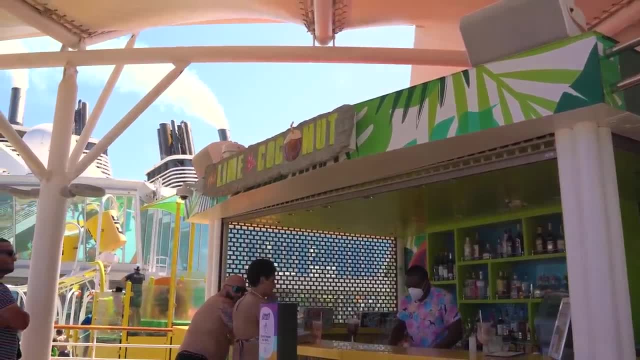 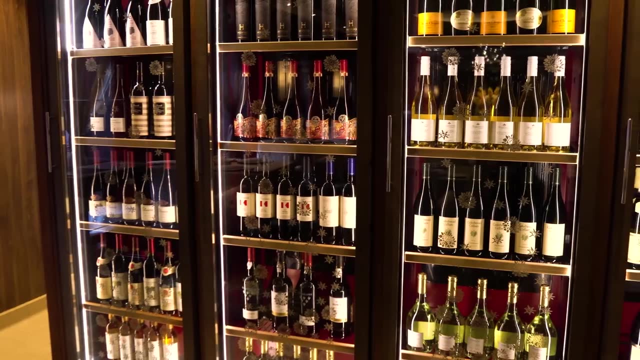 alcohol, and then there's also a soda package which includes just soda on board. There's a number of videos we've done about drink packages. Check those out for more information about that. Now, in addition to all that, Royal Caribbean does allow its guests to bring up to two bottles of. 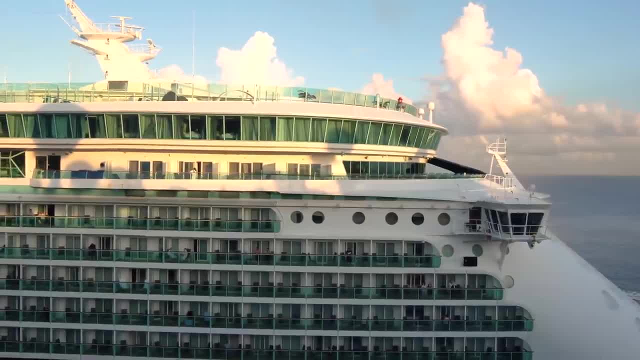 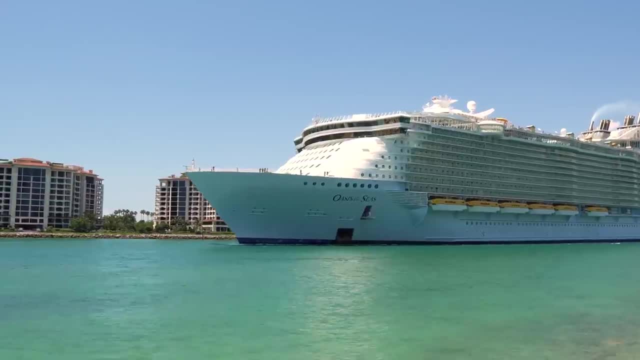 wine per stateroom with them on board on embarkation day. It must be brought on board on embarkation day and is subject to a corkage fee if opened in a public venue. You're also allowed to bring a limited amount of non-alcoholic beverages with you on embarkation day, Specifically: 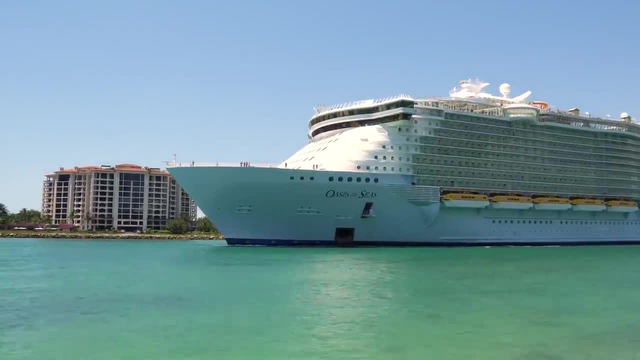 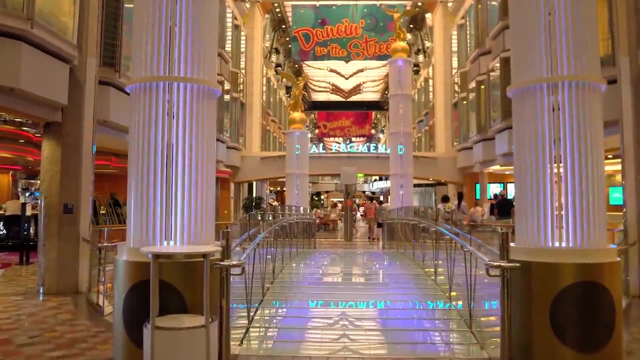 you can bring up to 12 standard 17-ounce cans or cartons per room of your favorite non-alcoholic beverage like soda, bottled water etc. but you can absolutely positively not bring on any hard liquor or beer on board your cruise. Now let's talk about room service, because room service on Royal 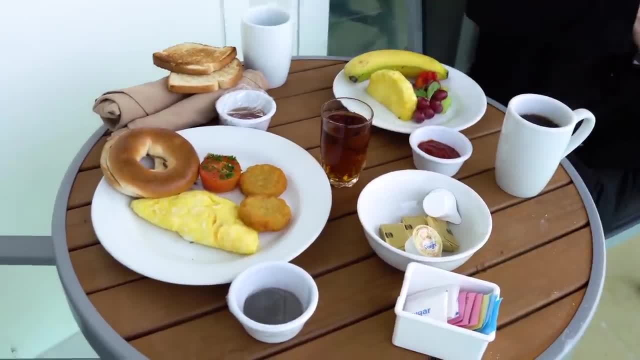 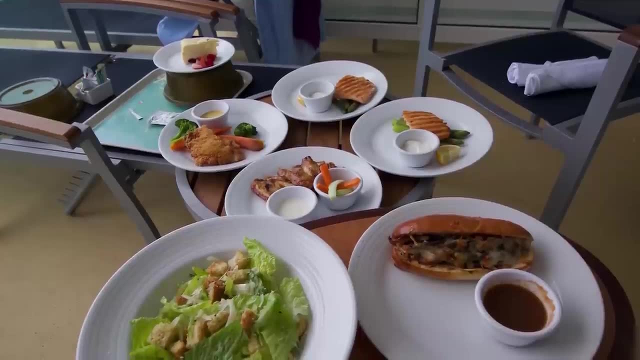 Caribbean is available 24 hours a day, but there is a $7.95 fee per order per room. As the fee is per room and not per person or per item, you can order as much as you like off the menu and only incur a $7.95 charge. There is, however, a continental breakfast option, which is a 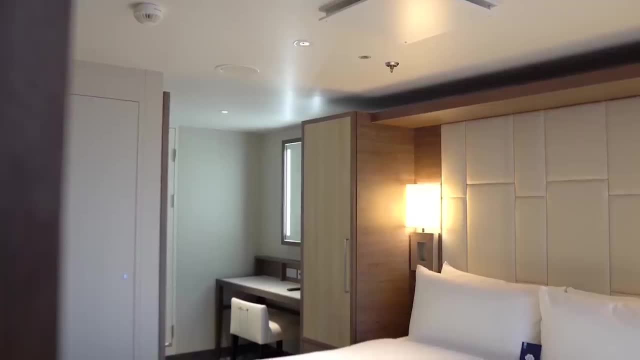 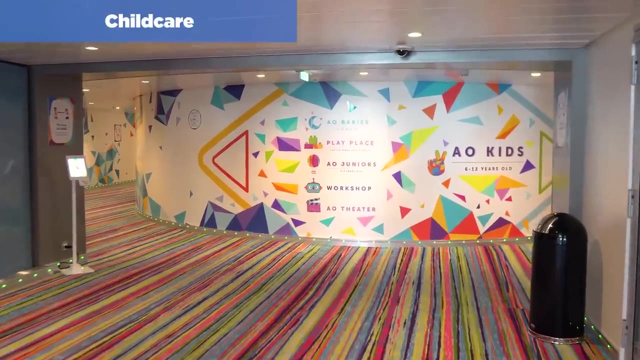 room service that is complimentary and doesn't have an order fee. Continental breakfast includes items like toast, yogurt, fruit, coffee and oatmeal. Next up is child care on board. Royal Caribbean's Adventure Ocean program is complimentary for children between the ages of 3 and 17 years. 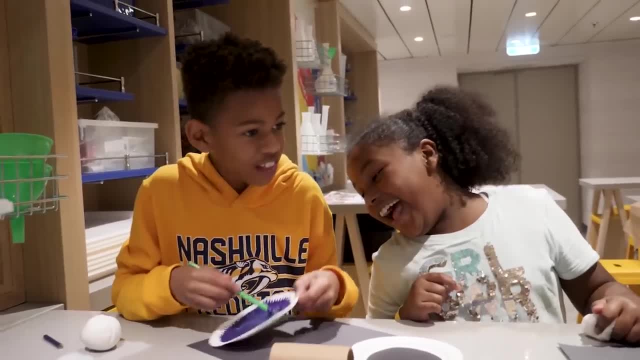 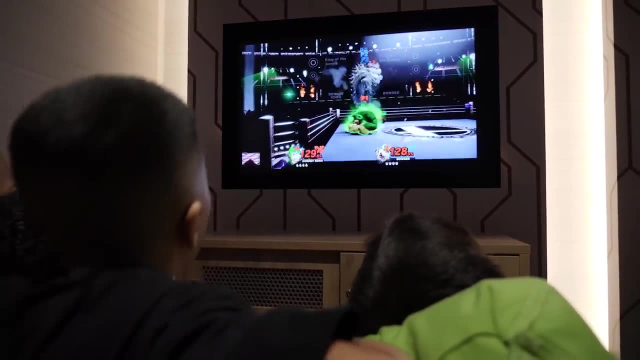 old. From when Adventure Ocean opens each day until 10 pm, there is no additional cost. From 10 pm to 2 am, Adventure Ocean incurs an hourly cost. While in Adventure Ocean, kids take part in activities led by the staff, There's lots of. 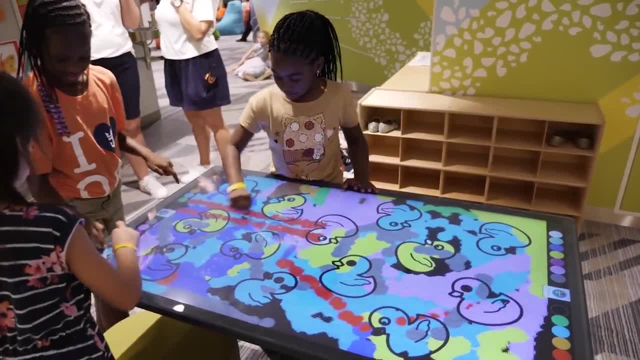 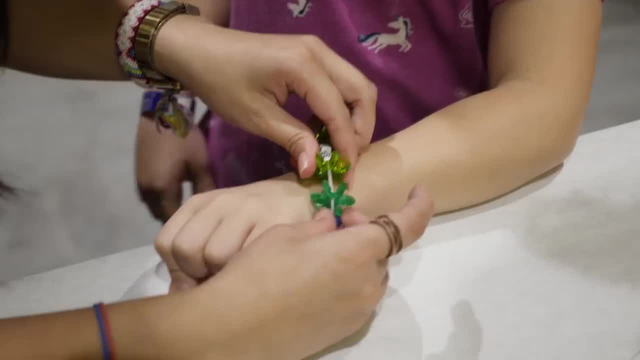 kids to do in Adventure Ocean and the programming is specialized for each age group. It's a mix of learning, playtime and socializing. Select ships have science labs and craft workshops in Adventure Ocean and these are led by the staff members with science, experiments and crafts and fun things to. do? Teens that are between the ages of 12 and 17 years old have access to a complimentary teen club and hangout area on their ships as well. Now, if you've got younger children between the ages of six months and 36 months old, they can participate in the Royal Babies in. 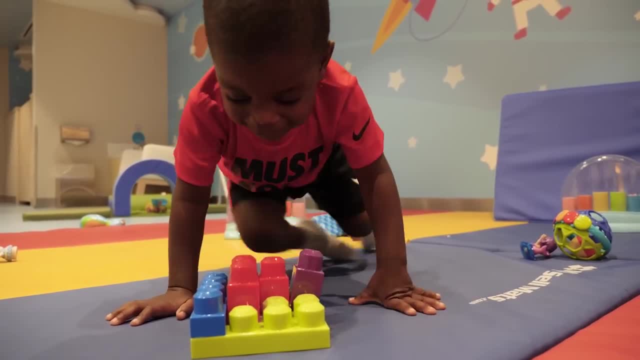 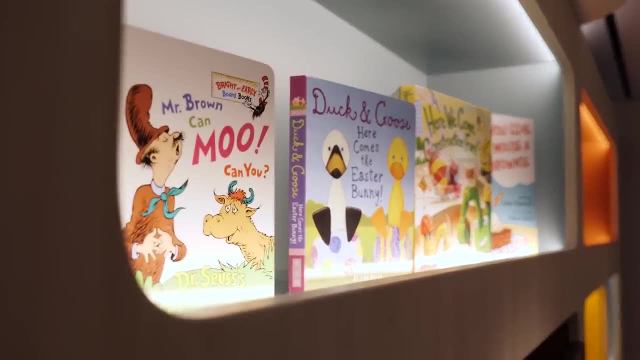 program. Most Royal Caribbean, but not all of them. most Royal Caribbean cruise ships offer a nursery where parents can drop their children off throughout the day and evening, but the use of the nursery comes at an hourly charge, All right. next up is activities and shows What entertainment is. 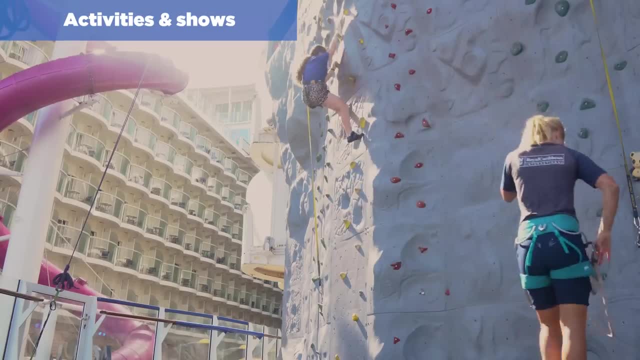 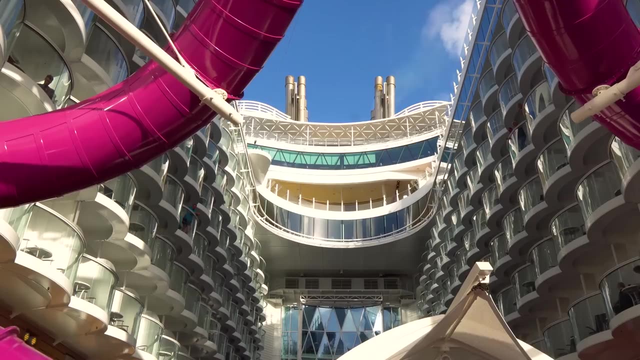 included with your cruise. A vast majority of the cruise activities that you're going to find in your cruise are going to be included with your cruise fare. Your daily cruise compass or the Royal Caribbean app will list a schedule of activities offered on board, and most have no. 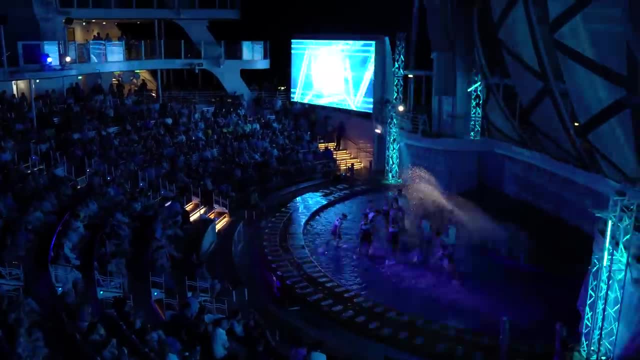 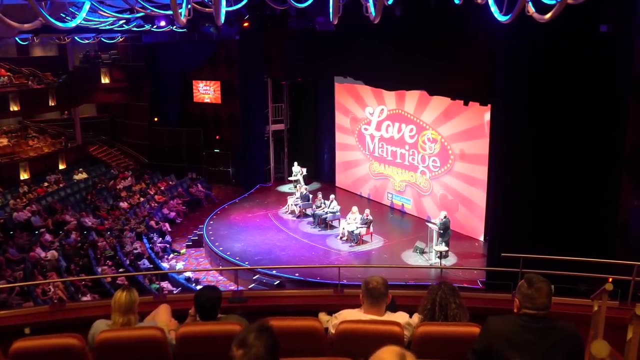 charge at all Performances in the Royal Theater, as well as the Aqua Theater and Studio B, are all included with your cruise fare. Likewise, comedy shows, magic shows, live music, audience participation shows and more are included as well, Even the Broadway shows that you 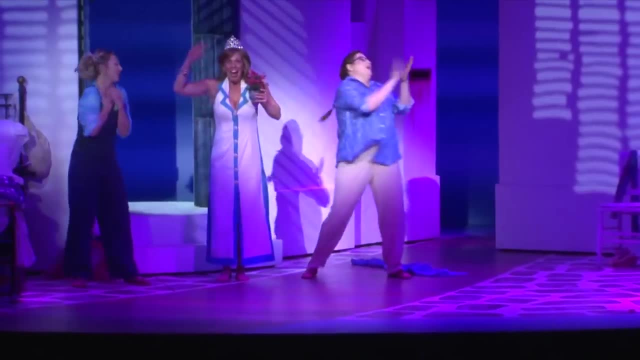 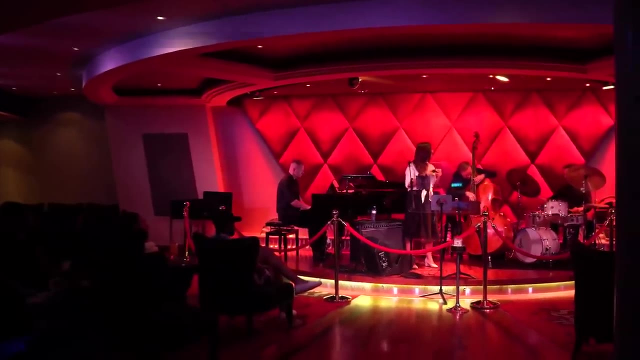 can find on. Royal Caribbean cruise ships are included with the price of your cruise, which is absolutely amazing. There will be shows each evening, along with additional performances throughout the day on sea days. Live music is also included with your cruise fare, which comes in many genres. 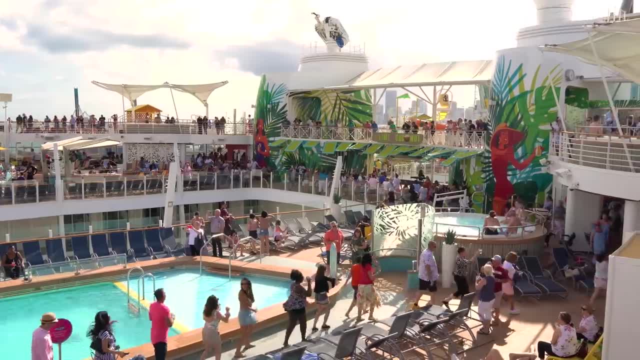 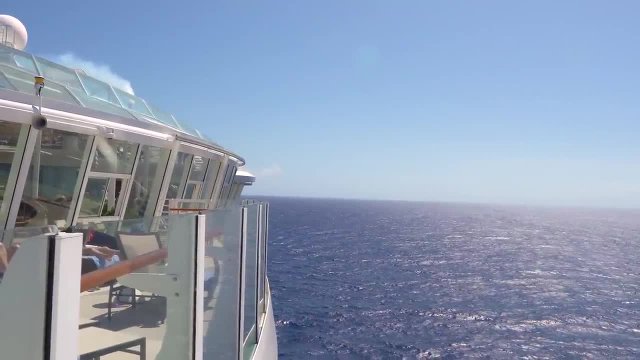 as it's often throughout the day, and multiple locations on board. Other activities like pool games, movies, trivia, dance classes and more are included with your cruise fare. Scavenger hunts are regularly offered on Royal Caribbean and have no additional charge There. 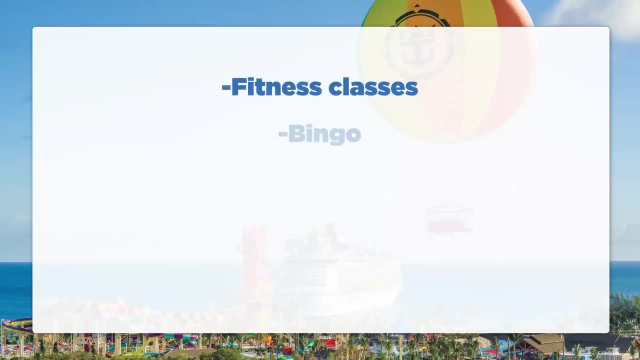 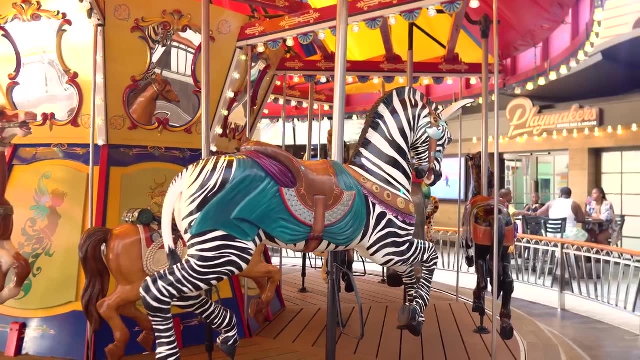 are some activities that have an additional fee, like fitness classes, bingo, anything in the casino, drink, seminars, spa services and more. Now, of course, the Royal Caribbean cruise ship probably has a signature activity and game on board, or both, and Royal Caribbean has some really. 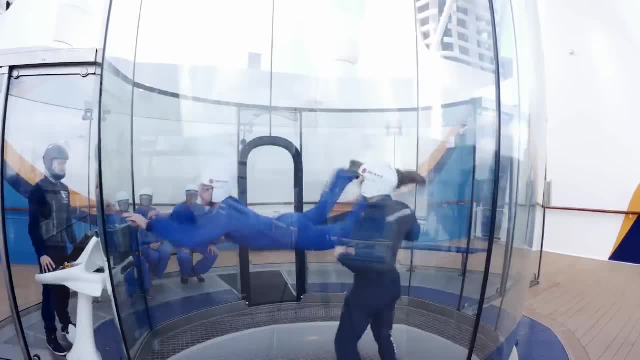 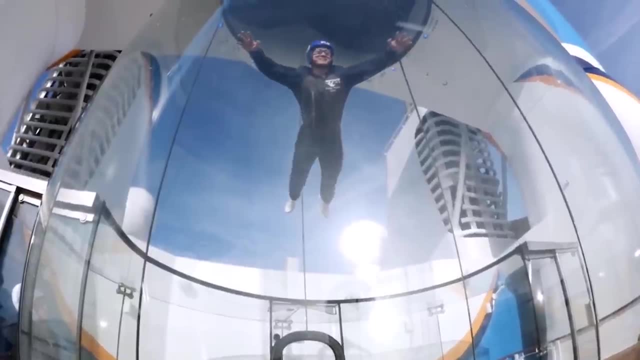 incredible things on board, and a majority of which are included with your cruise fare. If you watch any Royal Caribbean cruise commercial, you'll inevitably see people tackling the floor, rider, rock climbing and more In a skydiving simulator and more signature activities including your cruise fare include. 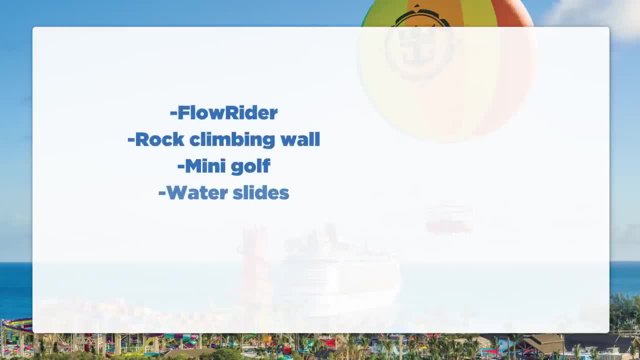 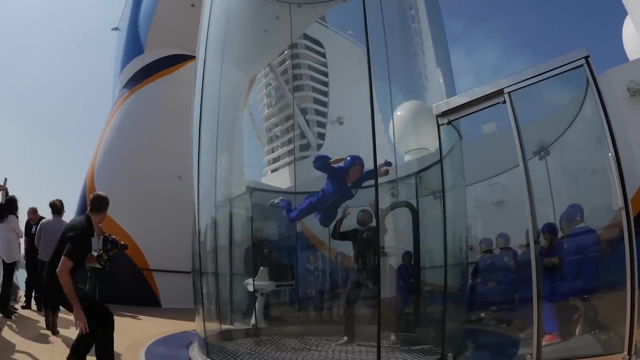 the floor rider, rock climbing wall, mini golf, water slides, zip line, ultimate abyss sports court, sea plex, bumper cars, aqua parks like Special Way Bay or H2O Zone, and ice skating. Ripcord by iFly, which is the skydiving simulator found on aquatic ships, has both complimentary. 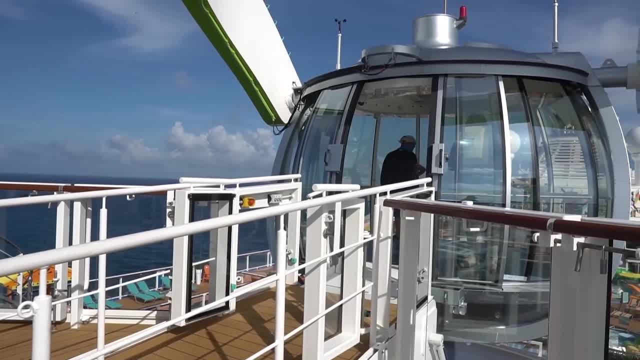 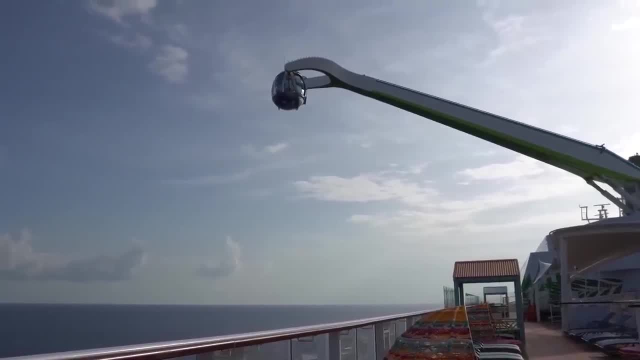 and extra cost options. Ditto as well for the North Star Observation Pod. Again, depending on if you're a sea day or a port day, there may or may not be an additional fee If you're a port day, but in general you can usually find at least one opportunity to go on it for no additional cost. 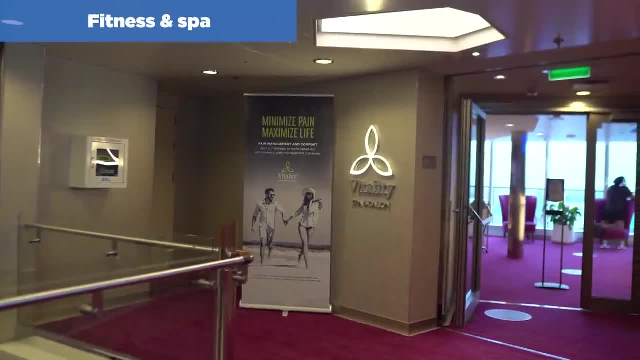 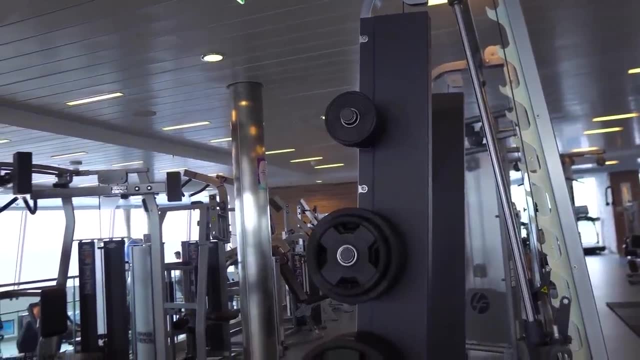 but they do have extra cost rides as well. Next up is the fitness and spa. Every Royal Caribbean cruise ship has a fitness center that offers cardio and weightlifting machines, free weights and more for no additional cost. Some, but not all, fitness classes are included in your cruise fare, such as stretching and ab. 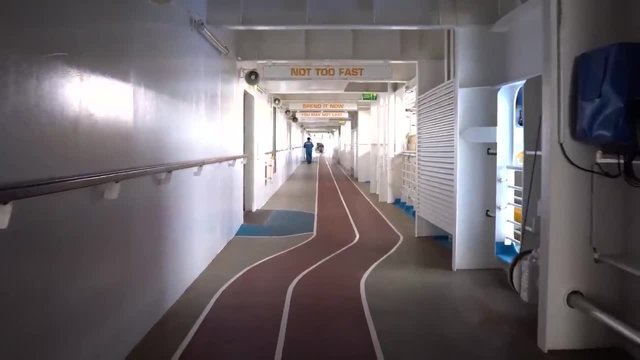 workouts. Every Royal Caribbean cruise ship also has a jogging track which is available to use throughout the day at no additional cost. The sports court, often referred to as the Garmin, is on the day at no additional cost. the sports court, often referred to as the c-plex on quantum class ships. 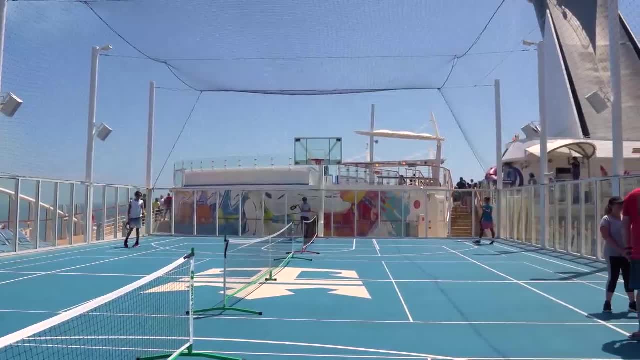 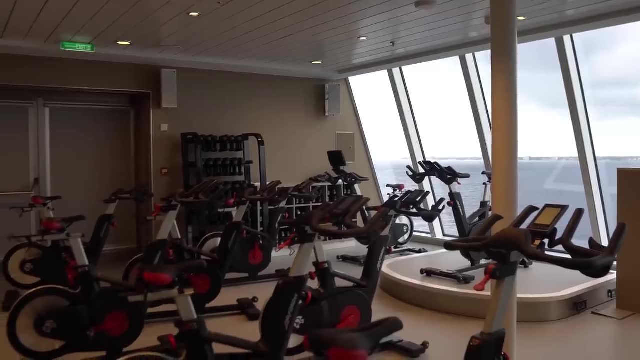 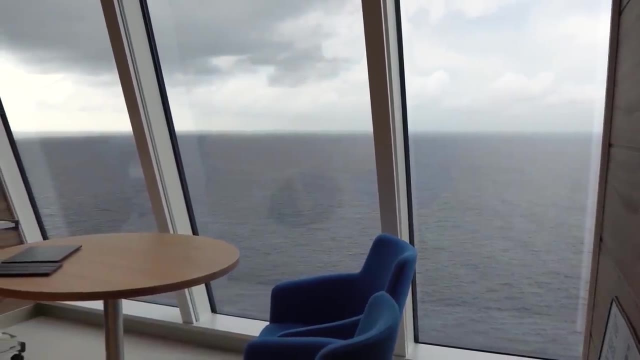 also offers complimentary use of its facilities with organized sport games to help throughout the sailing. outside of the few select fitness classes, including your cruise fare, the fitness center offers extra fee classes for yoga, spinning, pilates and more. the fitness center also offers personalized training and consultations that have an additional fee. the spa is not included in your. 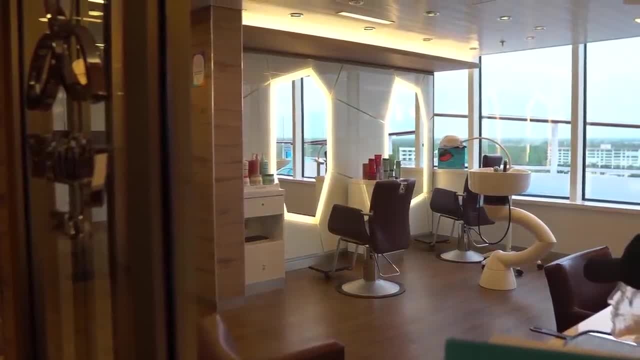 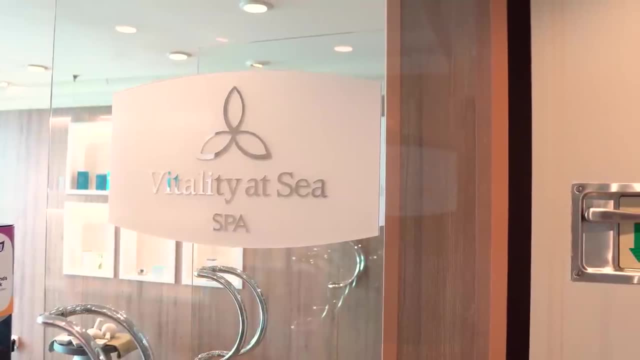 cruise fare at all, and spa treatments, salon services and day passes all come with an additional cost. some royal caribbean cruise ships have a sauna, hot tub and or steam room available at no additional cost, but again it depends on the ship you're sailing on, and some ships have a thermal. 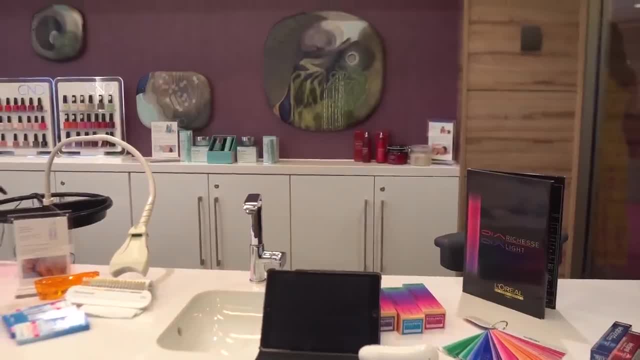 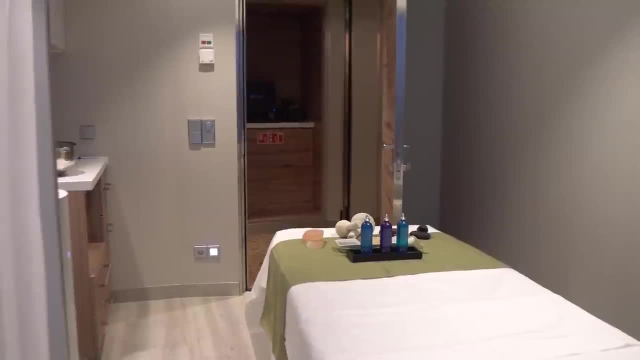 spa, of which you can purchase a pass, for tours of the spa are available at any time during your cruise and they have no additional cost or obligation. in fact, these tours are a great way to learn about what the spa offers. if we head outside, access to royal caribbean's pools are 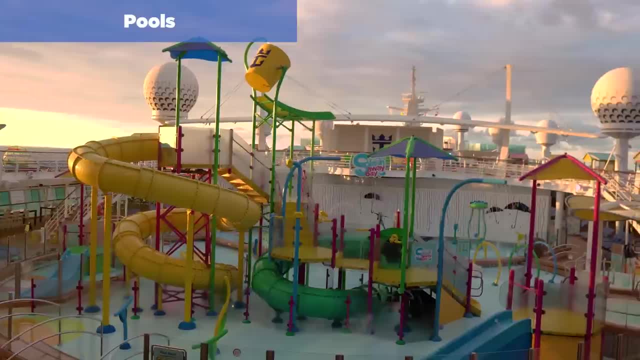 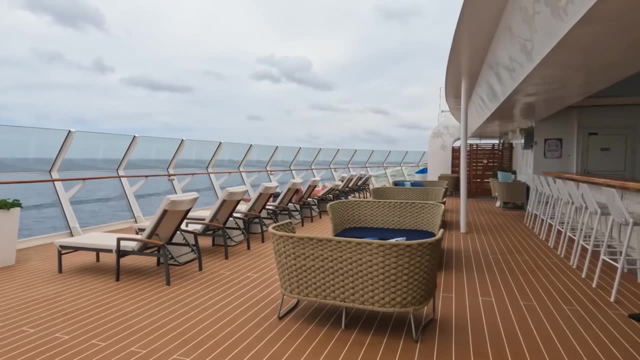 included with your cruise fare, including lounge chairs, hot tub, water slides, aqua parks and more. the solarium area, which is the adults only pool area, also has no additional cost, but is limited to adults only. some of the areas of the pool deck are reserved for suite guests. only if you're a suite guest, which is a grand suite and above, you'll have 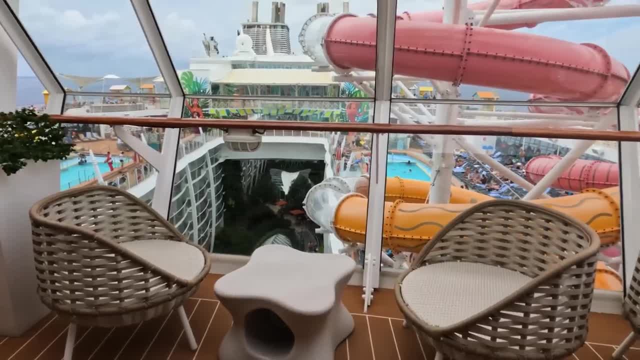 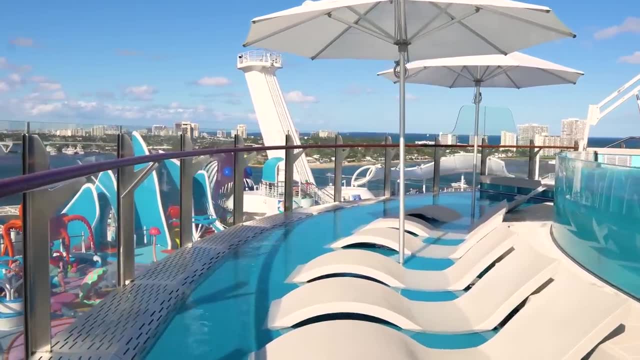 access to complimentary access to these areas and depending on the ship, the suites only area can be a small section of reserved lounge chairs or an entire deck area. wonder of the seasons, as an example, has an entire suite neighborhood dedicated to suite guests, with its own pool, bar, outdoor. 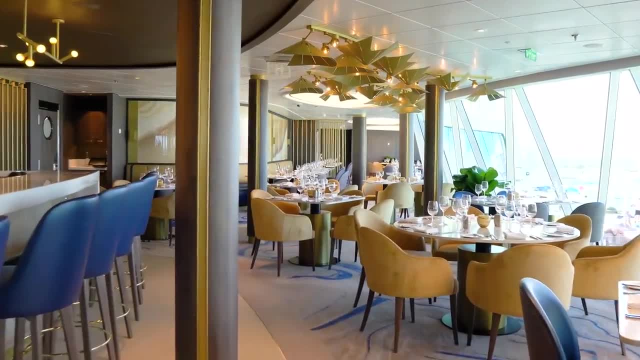 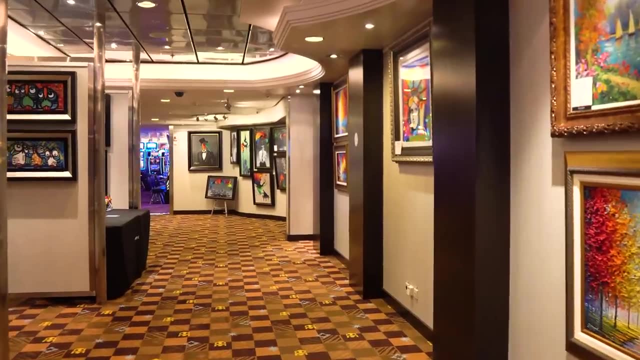 hangout area, lounge and restaurant. now, in terms of other things that just don't fall into any category we talked about, there are some other things that are not included with your cruise fare, such as gambling, including bingo, art auction, any purchases made in the gift shops on board shore excursions, photographs, video arcade.